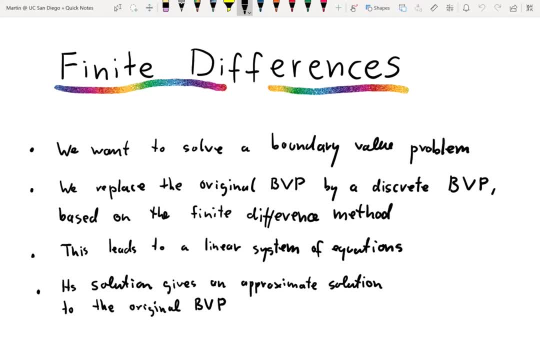 In this video we're going to develop the final difference method for a one-dimensional model boundary value problem. So let us discuss the broader perspective of how the final difference method is used. At the outset we want to solve some boundary value problem, maybe a 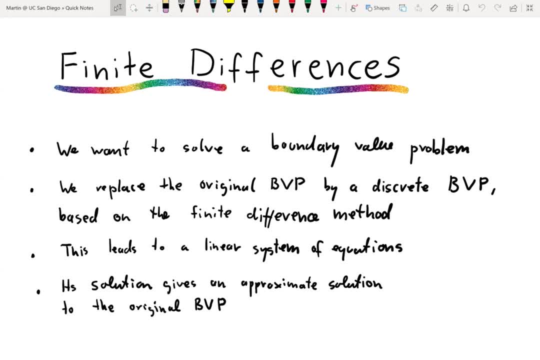 stationary equation, for example. The final difference method is a mathematical construction that in some sense replaces the original boundary value problem by a discrete boundary value problem. That discrete boundary value problem that we construct by the final difference method boils down at the end of the day, to a linear system of equations, which, of course, 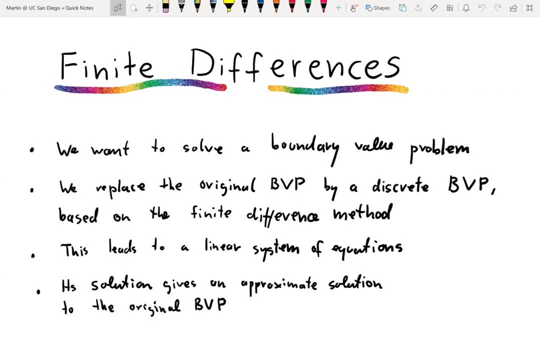 we can solve with techniques from numerical linear algebra. And while the solution to that linear system of equations is the solution to that discrete boundary value problem, the solution to the final difference methods of trying separate, say. That solution we use as an approximation to the solution of the 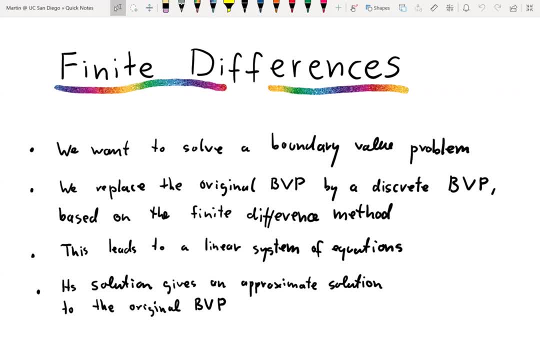 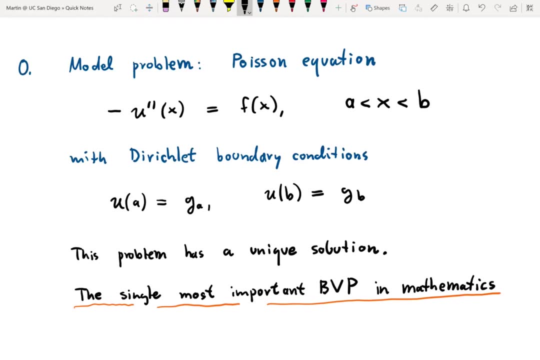 original boundary value problem. That is a broad agenda of what we're going to do. We are going to develop that with a concrete example. Step 0. We introduce a model boundary value problem, namely the so-called Poisson equation. The one-dimensional Poisson equation is a differential equation over an interval. 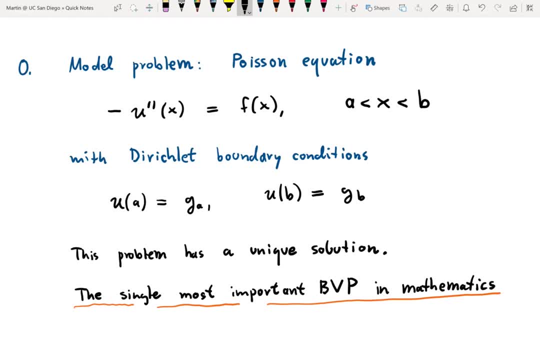 from a to b. It is the second order differential equation where the unknown function u satisfies negative u. prime prime of x, equal f of x. More specifically, we are going to consider the Poisson equation with Dirichlet boundary conditions, which means that we fix the boundary values of the function. 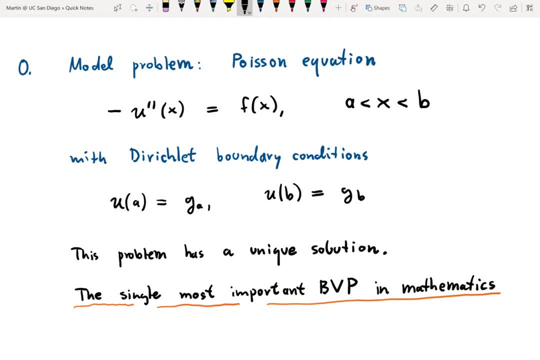 at the left endpoint of the equation. So we demand that u equals some number g and u equals some number g. The Poisson equation with Dirichlet boundary conditions is a boundary value problem and one can show that this boundary value problem has got a unique 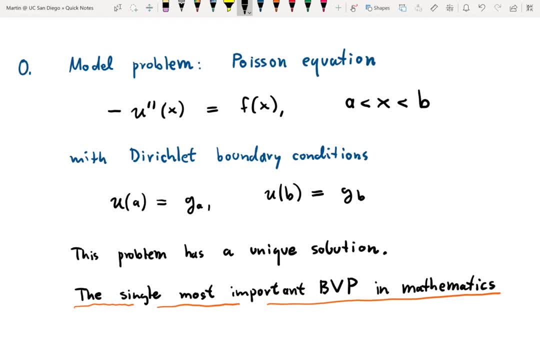 solution. In fact, the Poisson equation with Dirichlet boundary conditions is probably the most important一定 Abbcy thinker around F, But we can't actually possibly be�� in to P, so we're taking agreed Poisson equation with Dirichlet boundary. conditions and we're going to look at it from different angles. The one-dimensional Russian Basic equation that we use used phonetically what is a differential equation, and what Jennifer has to do is define the right final, irresponsible error that will result in a pair between the terms of the 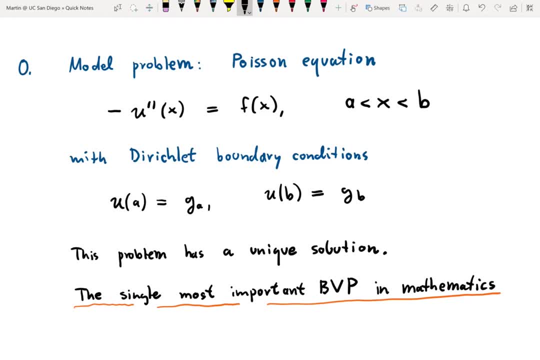 angle and the worth. these will leverage corresponding factors. model-value problem in all of mathematics. Even though it looks fairly simple, it is the most important model problem in all of numerical analysis. I'd say that probably 90% of all research publications in numerical analysis are to some extent concerned with the Poisson equation. 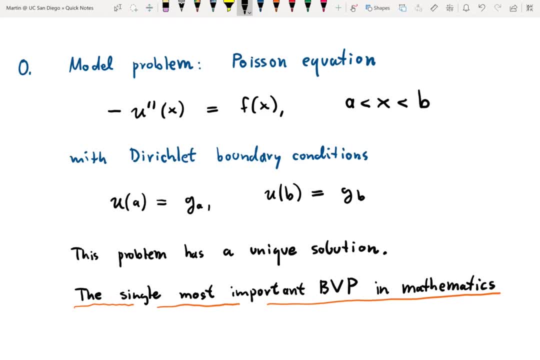 The reason is that the Poisson equation is fairly well understood and as soon as you go even slightly more general, then you easily find yourself in uncharted territory. Let us contemplate for a moment why, fårishly, boundary conditions seem to be a natural choice of boundary conditions. Let's suppose I've got a solution u of the Poisson equation. 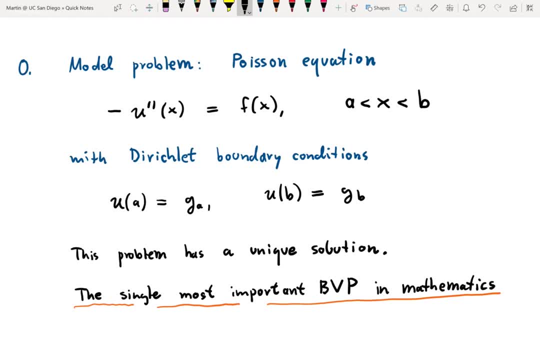 If I add some linear function to that solution u, then this new function will again solve the differential equation of the Poisson problem, because the second derivative of linear fucking law of space is 2. non- şeyi function vanishes. So it seems intuitive that the solution cannot be unique until I, unless? 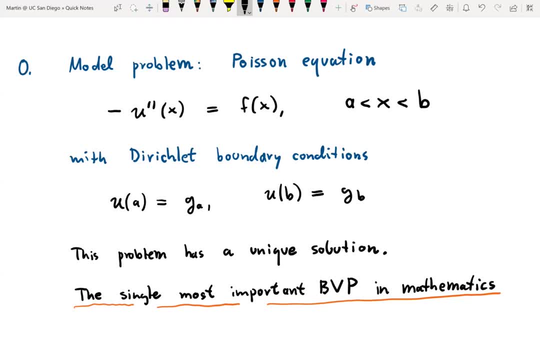 I make some additional requirements. In fact, since the linear functions are precisely those functions whose second derivative is zero, I only need to add two more conditions in order to make the solution unique- if the solution exists, of course, And one way of. 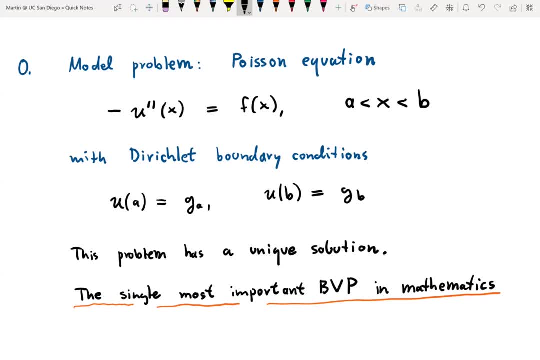 doing so is to set the boundary values of the function at the endpoints of the interval. Finally, let me also remark that this differential equation is also known as diffusion equation, Because with that simple second derivative equation you can describe diffusive processes in physics like, for example, the diffusion of heat, the diffusion of water in the soil. 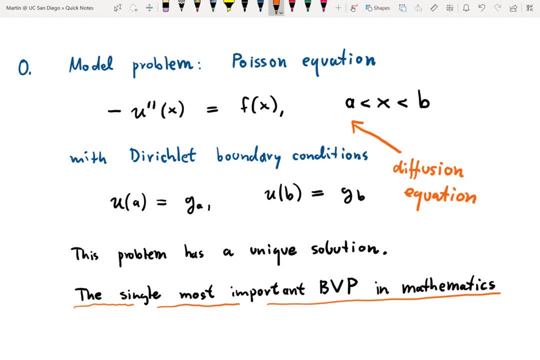 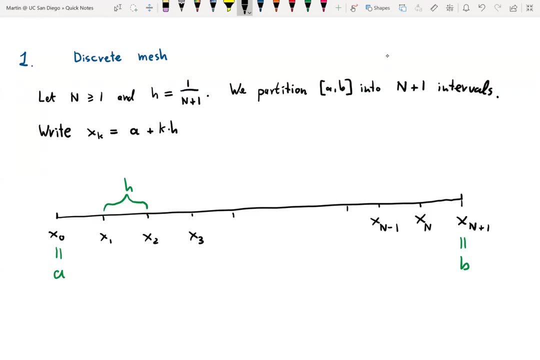 the diffusion of chemicals in water. maybe it's a diffusion of bacteria and liquid. This is one of the most universal differential equations you're ever going to meet in mathematics. That all being said, we are here for a discretization of the differential equation And the starting 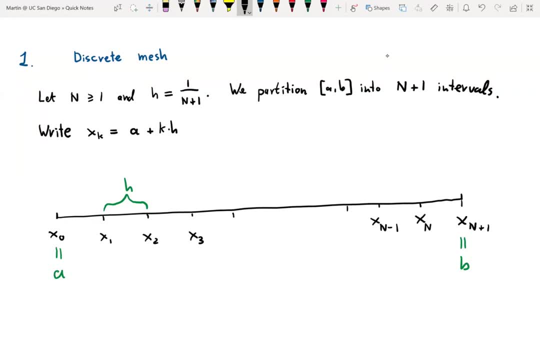 point for that is to introduce a discrete mesh over the interval from a to b. the interval of interest Let n be a number greater than 1, and let us define h as 1 over n plus 1.. We are going to partition the interval from a to b into n plus 1 subintervals, And each of the subintervals 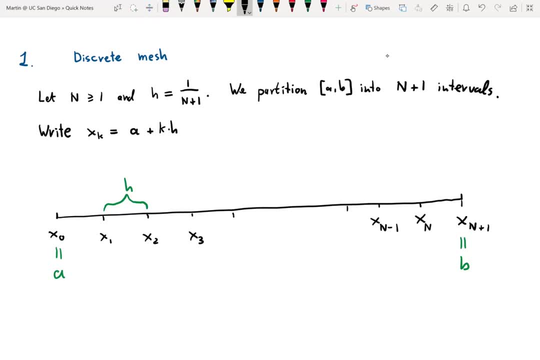 is going to have length h. The boundaries of the subintervals are nodal points Within the interval. let us define xk as a plus k times h. So we go k steps of size h, starting at the left boundary of the interval. 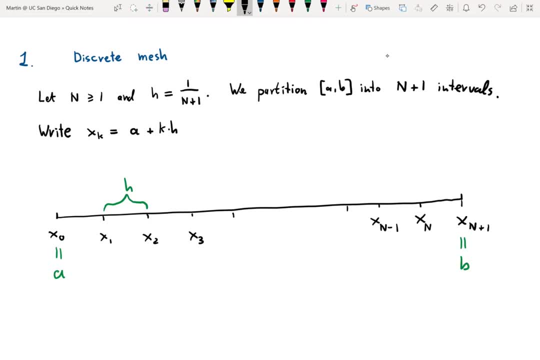 In this partition, the left endpoint a equals x0,, the next point is x1,, the next one is x2, up to x3, and so on. The difference between consecutive nodal points is always the step size h. Eventually we come to xn minus 1,, xn and finally xn plus 1,, which is the right endpoint. 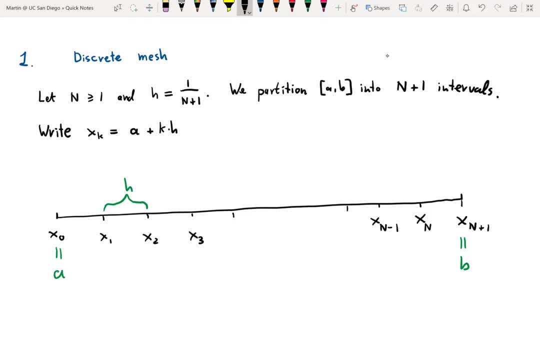 of the interval called b. The nodal points x1, x2, up to xn are the interior nodal points of the interval and x0 and xn plus 1 are the boundary nodes. We call the collection of nodal points a discrete mesh. 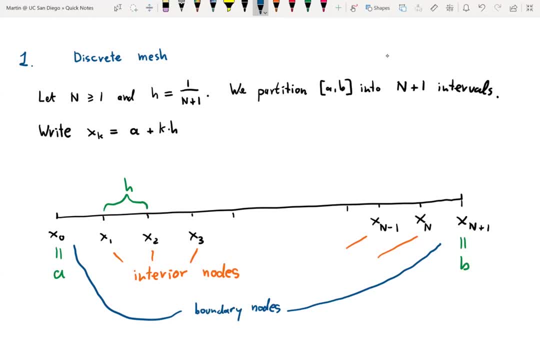 Okay, so what is the point of this discrete mesh? The point of that discrete mesh is as follows, namely, we are going to approximate the solution u to the original boundary value problem at the point x0,, x1,, x2, up to xn plus 1.. 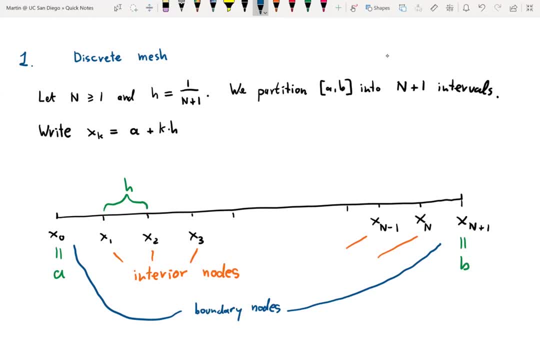 We're going to introduce the new boundary node and we call the discrete node m at xn plus 1.. We call the discrete node for the situation, We call the discrete node for the solution from the point x, y to 1,, xn plus 1, and. 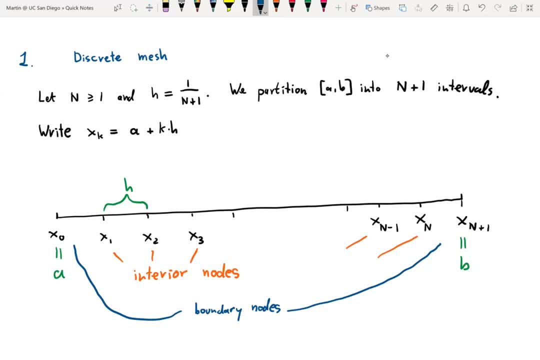 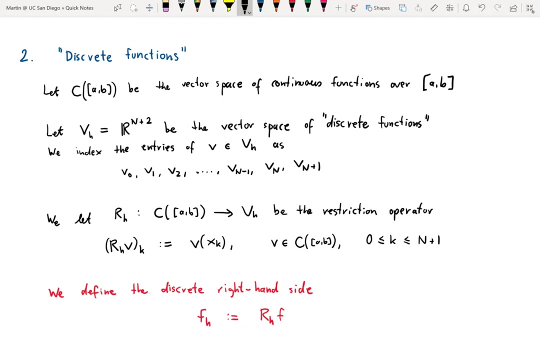 Just like we approximated the solution to an initial value problem at different points in time, at different time steps, we are going to approximate the solution of a binary value problem at different points in space. In some sense, the discrete mesh defines a discrete geometry, so to speak. 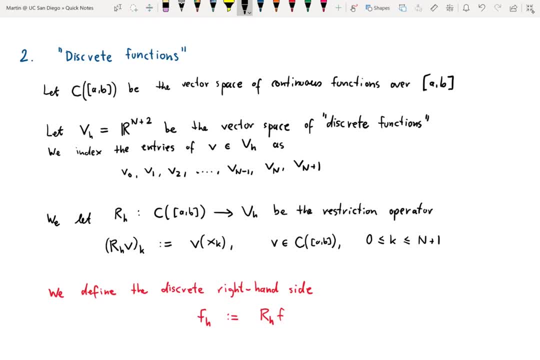 And on this discrete geometry we develop a notion of what you might call discrete functions. However, much of this slide is mostly notation. It is not particularly deep, but establishing that notation is going to help us to understand the finite difference method, which will be complicated enough. 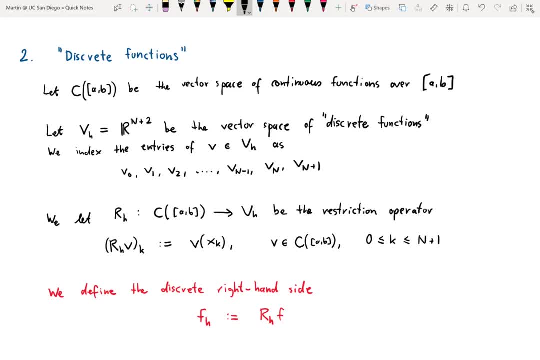 So, to begin with, we recall that c is a common notation for the vector space of continuous functions over the interval from a to b. Furthermore, let us define the vector space vh, where h is a step size as r to the n plus. 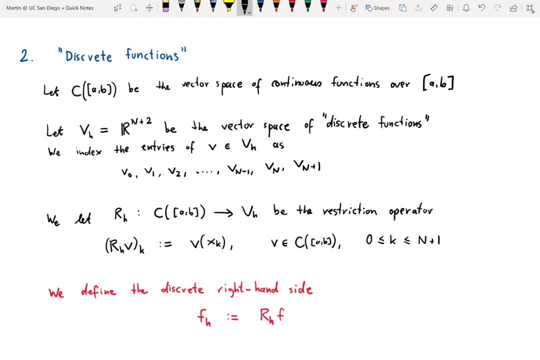 2, where n is the number of interior nodes, just as in the previous slide. So that is just the Euclidean vector space of dimension n plus 2.. Conceptually, this is going to be a vector space of discrete functions, Which of course is a very ceremonial term for something very simple. 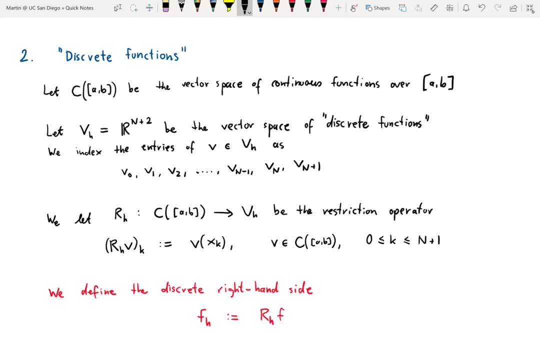 So what is the Euclidean vector space? It is going to be the vector space of an integral function. This is going to be the vector space for the function, which is, of course, a very ceremonial term for something very simple. We are going to index the entries of the vectors in vh by v0, v1, v2, up to vn-1, vn, vn-1. 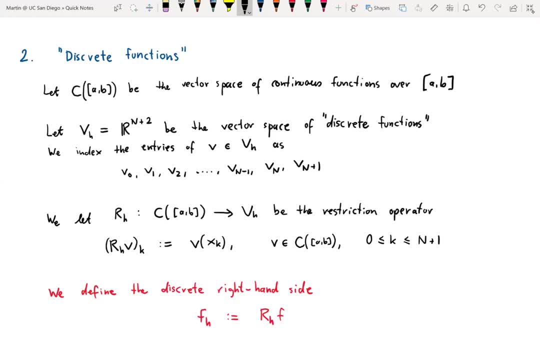 So if v is an element of vh, then the coordinates of v in some sense give us the values that we associate with the nodal points of the discrete mesh. It could also be helpful to establish a restriction operator. So we define the mapping rh as the linear mapping that goes from the space of continuous 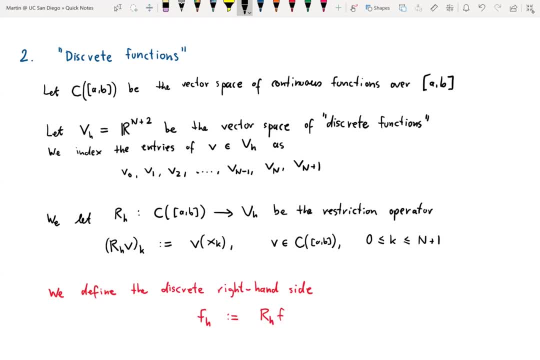 functions over ab into this vector space, vh. This mapping can be described as follows: If v is a continuous function over ab, then the kth entry of rh- the kth in between 0 and n plus 1, is defined as v at the. 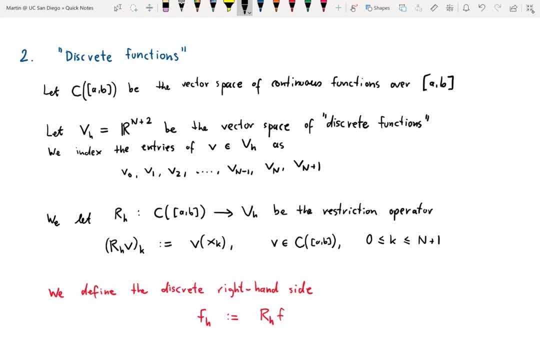 nodal point xk. So to put it into somewhat simpler terms, we take a function v that is continuous over ab, and then we sample that function over the nodal points x0, x1, up to xn, xn plus 1.. 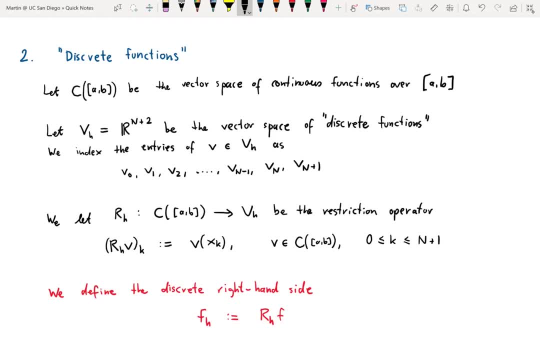 And these samples of function values of v are then put into a vector. That vector is rh. In fact we are going to do that with the right-hand side of the boundary vector. So we define fh as rh. In other words, we take the function f, then we sample the values of f at x0,, x1, up to 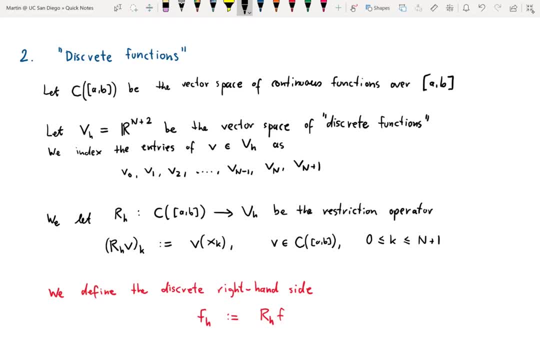 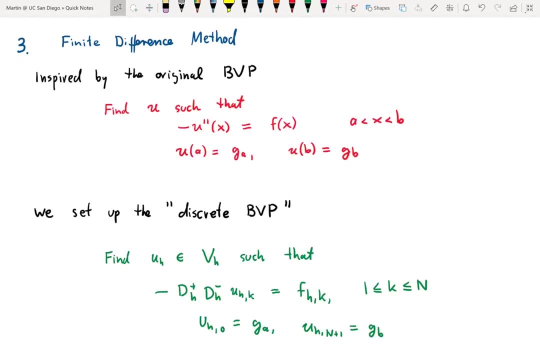 xn plus 1, and put this into a vector which we call fh Again. this is just lots of notation, And now everything is in place to get started with the finite difference problem. The starting point for the finite difference method is, of course, our original boundary. 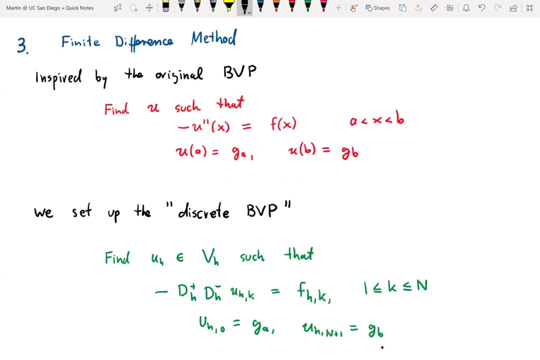 value problem, where our goal was to find a function u such that negative u' of x equals f for all x between the interval boundaries a and b, And then, together with the Dirichlet boundary conditions, u of a equals ga and u of b equals. 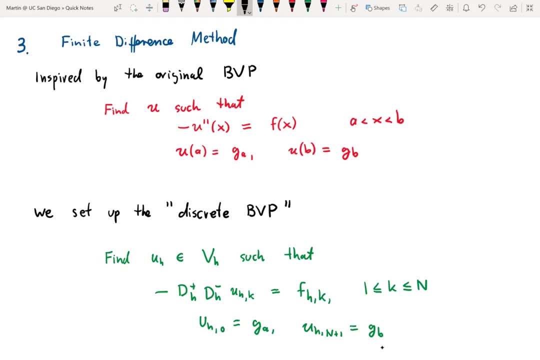 gb. The idea of the finite difference method is that we replace this original boundary value problem by a discrete boundary value problem. The right-hand side, f, is then a discrete function from the space vh, and also the unknown that we seek is an element of the discrete function space. 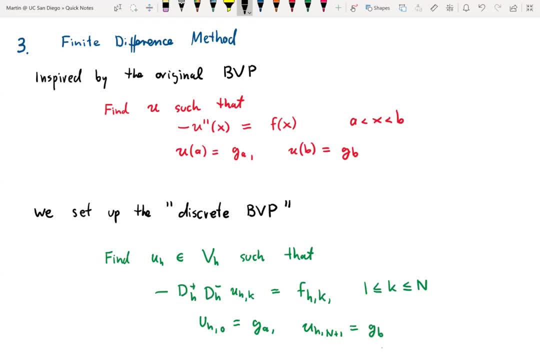 And the derivatives in the differential equation are replaced by difference quotients Which, as we have already marked, are in some sense discrete derivatives. So the discrete boundary value problem that we get in the end is searching for a vector uh from the space vh of discrete functions, so to speak, which satisfies the differential. 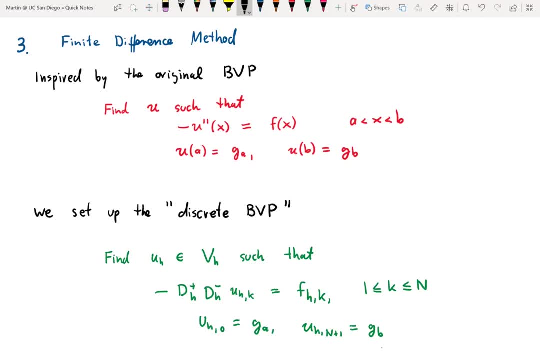 equation: negative forward difference with step size h of the negative backward difference with step size h of uhk. And so what we are doing is that we are turning the parameter curve over to u of vh And to further done, we are calculating definition and simplification for u of u of vh. And from this we can now compute the expression f of vh. Or for a general equation we can say: u of u of vh is equal to fhk, where k is an index of an interior node. K is between 1 and n. And furthermore we've got uh0 equals ga and uhn plus 1 equals gb, which are just the discrete analogs of the boundary conditions. It is probably helpful to be more explicit here. This is the classic example of the derivative problem where u of u a equals fhk and u of u a equals. 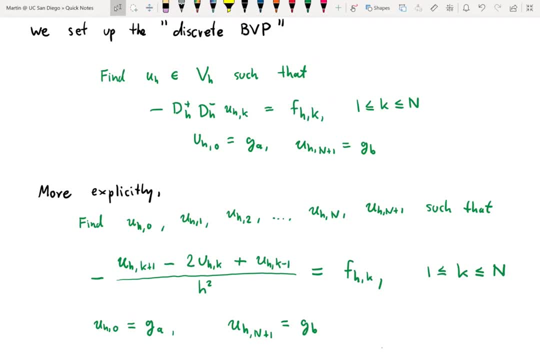 a. In some sense we are looking for entries UH0,, UH1,, UH2, and then further and further up to UHn, UHn plus 1, such that for all k between 1 and n we have got this discrete. 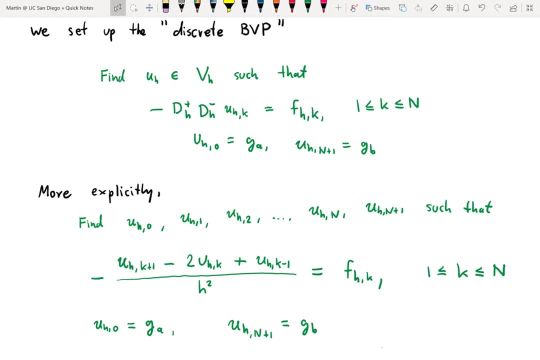 differential equation at index k, namely negative of the second-order difference quotient: UHk plus 1 minus 2 times UHk plus UHk minus 1, divided by h square equal fhk. And then we have got the discrete boundary conditions: UH0 equals ga and UHm plus 1 equals. 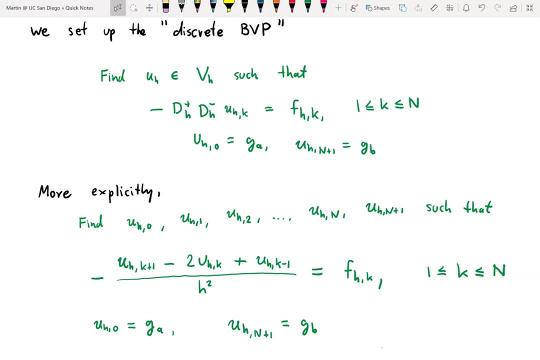 gb. So if we take all these values- UH0,, UH1,, UH2, and then we have got the discrete boundary conditions UH1 up to UHm plus 1, and put them into a vector and call that vector UH, then 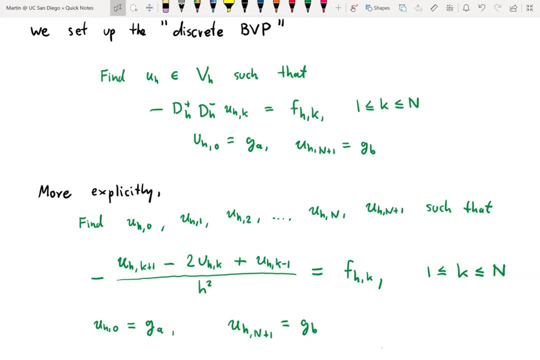 what we get is an element of vh, a discrete function, so to speak, that is defined at the nodal points of the discrete mesh, And these entries of the vector UH are approximations of the function. u are supposed to be approximations. 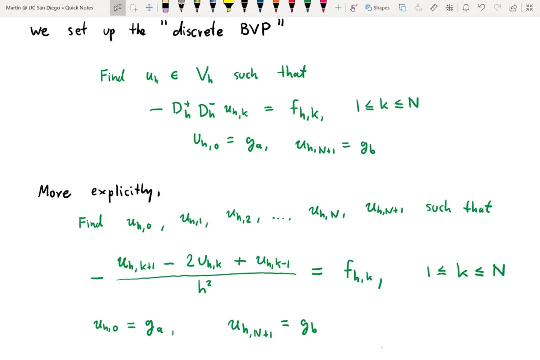 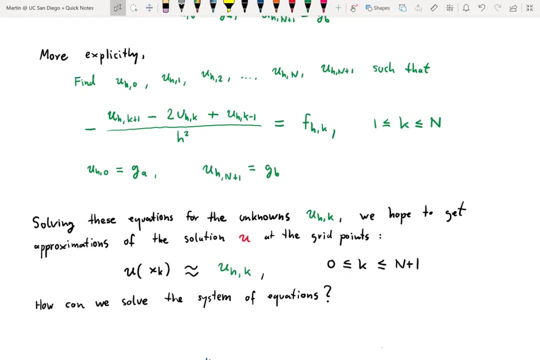 of the original solution u at the nodal points. So we have got several equations in n plus 1, variables indexed from 0 to n plus 1.. And if we solve these equations for the unknowns UHk, then we hope that we get reasonable approximations. 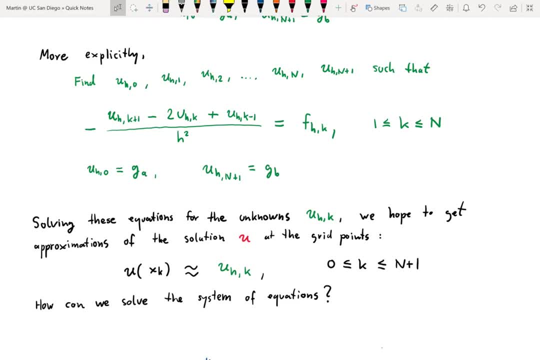 to the solution: u at those grid points, which means u at the grid point Xk is supposed to be approximated by UH, indexed from 0 to n. So we have got several equations in n plus 1 variables indexed from 0 to n plus 1.. And 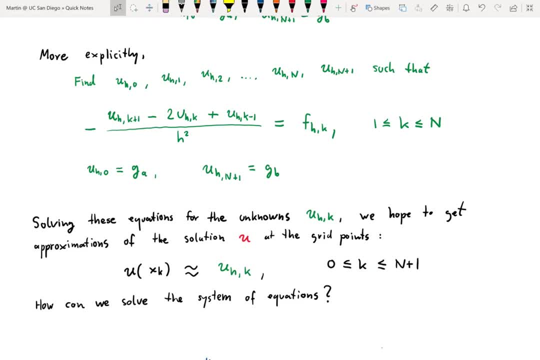 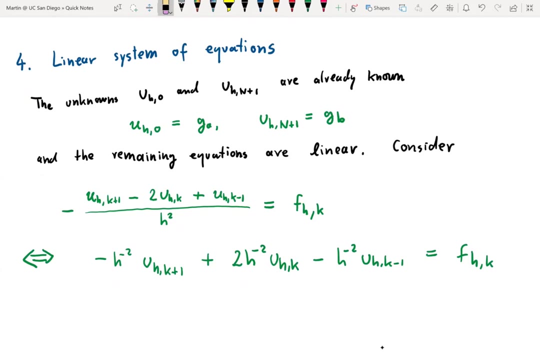 xk. Okay, now we are left with a purely discrete problem, namely, we have several equations and we have got n plus 2 variables. How can we solve the system of equations Now? we can easily notice that these equations in fact define a linear system. 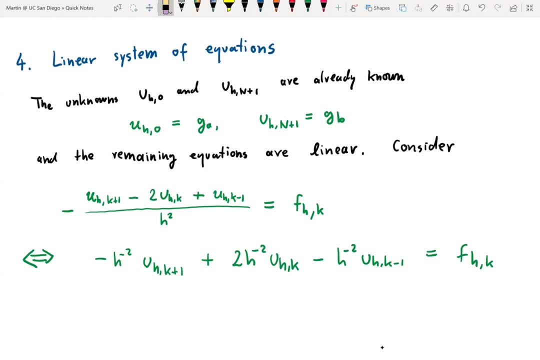 of equations. Linear systems of equations is very good, because then we are just in the domain of linear algebra. Okay, first we notice that the unknowns uh0 and uhn plus 1 are already known, which is, I think, quite obvious. uh0 is equal. 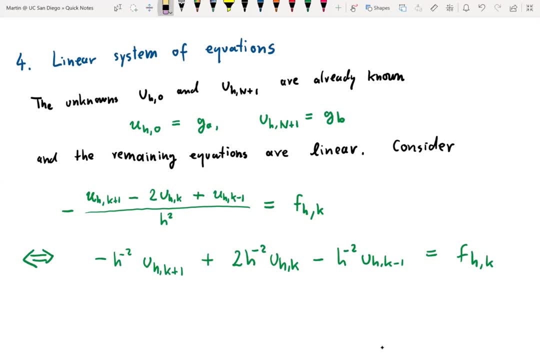 to ga and uhn plus 1 is equal to gb. Yet now all the other remaining equations involving the variables uh1, uh2 up to uhn are in fact linear equations. So if we consider the equation that's associated with the grid, point k negative of the fraction uhk plus, 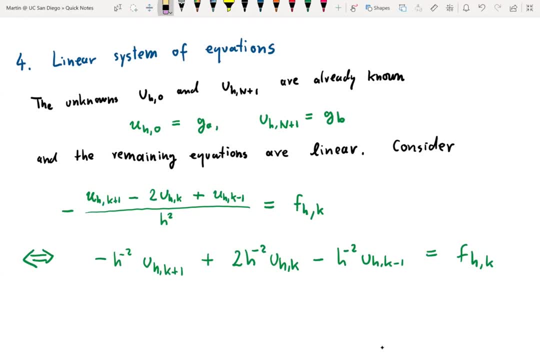 1 minus 2 times uhk plus uhk minus 1, divided by h square, equal fhk. then of course we notice that this is a linear equation in three variables. If we factor everything out, what we get is negative h to the minus 2 times uhk plus 1. 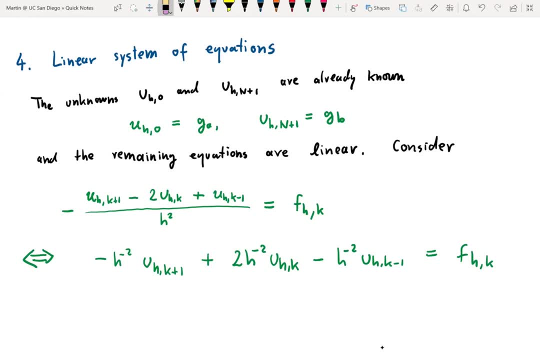 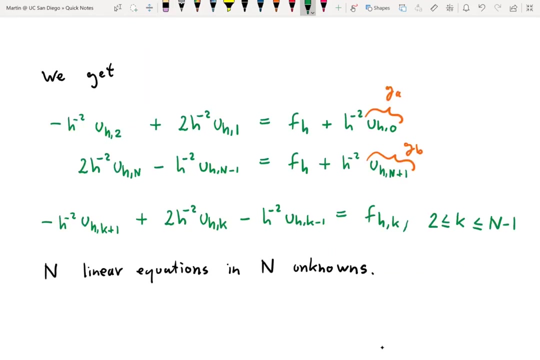 plus uhk minus 1.. That means 2 times h to the negative, 2 times uhk minus h to the negative, 2 times uhk minus 1 equal fhk. So the variables uh nought and uh nought are already known. they equal gA and gB respectively, and so we are left with n equations and n. 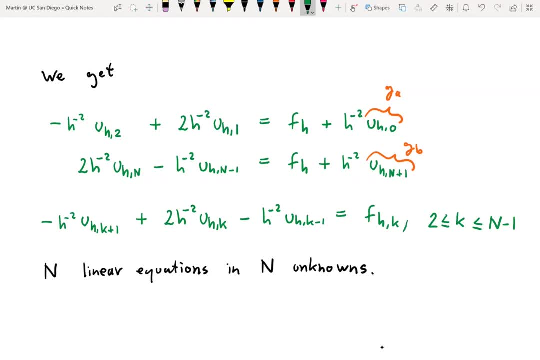 unknowns. The equations are associated to the interior mesh nodes, to the interior nodal points, and the unknowns are precisely the values of UH at the interior nodal points, UH1, UH2, up to UHm. In other words, we can assemble a linear system of equations with 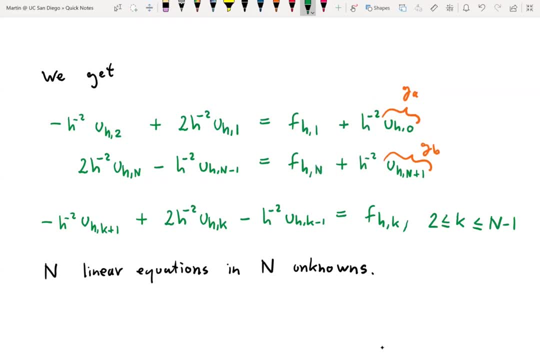 n unknowns and n equations. Specifically, plugging in the values for UH0 and UHm plus 1, we get the equation negative h to the minus 2 times UH2 plus 2 times h to the negative 2 times UHm. 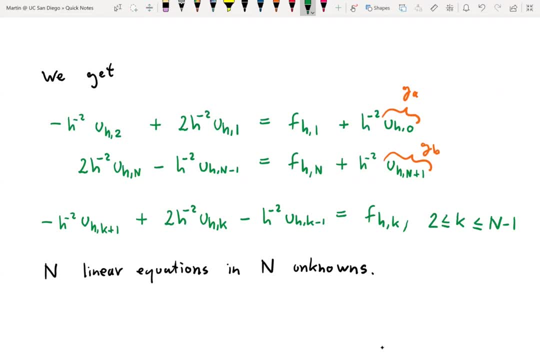 UH1 equal fH plus h to the negative, 2 times gA UH0.. Then we have 2 times h to the negative, 2 times UHm minus h to the negative, 2 times UHm minus 1 equal fHn plus h to the negative. 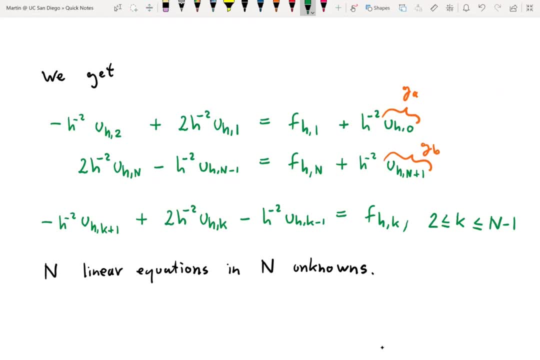 2 times UHm plus 1, which is gB, And then for all the indices k between 2 and n minus 1, we get negative h to the negative 2 times UHk plus 1 plus 2 times h to the negative, 2 times UHk minus h to the negative 2 times. 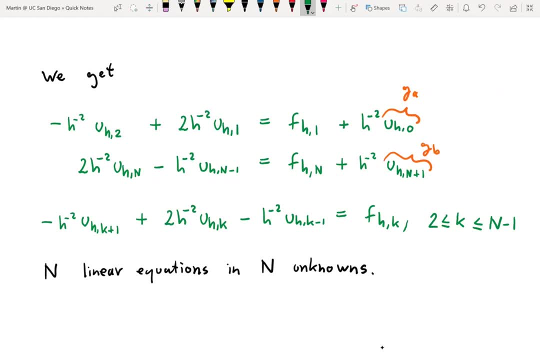 UHk minus 1 equal fHk. The first two linear equations here are associated with the mesh points X1 and Xn respectively, and they look a bit different from the other ones because the boundary values are right next to them, because they're influenced by the boundary values. 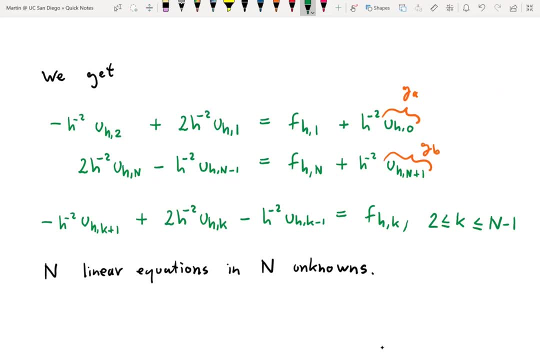 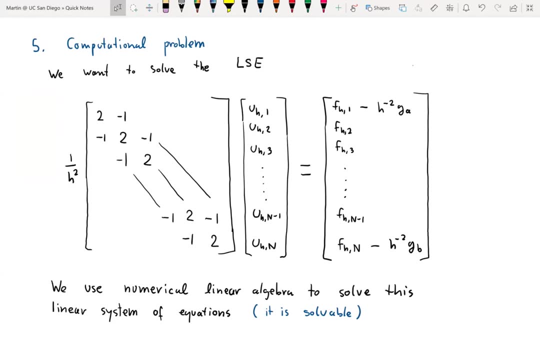 at x0 and xn plus 1 respectively. As you know from linear algebra, often it's quite helpful to put a linear system of equations into a matrix form. So the computation problem- that's a final difference method for our boundary value problem- boils down to 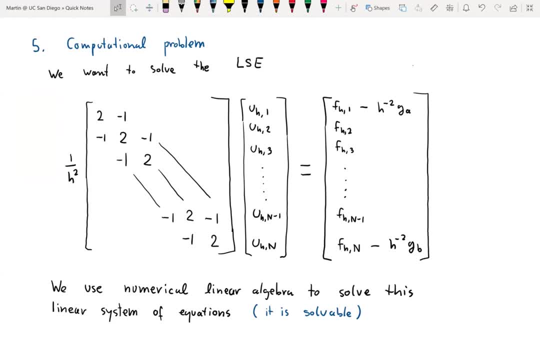 is a huge linear system of equations with the following matrix and the following right-hand side. Let's take a look at the right-hand side first. The right-hand side has n entries. The first one is fh1 minus h to the negative, 2 times ga. 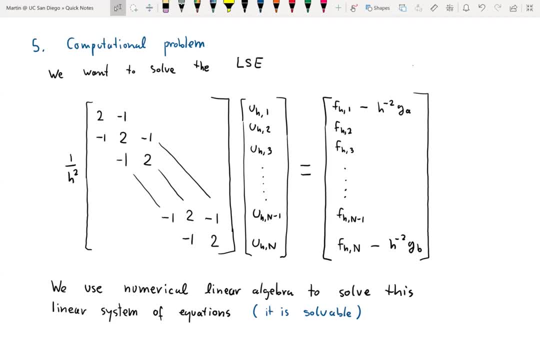 The last one is fhn minus h to the negative 2 times gb, And all the ones in between are the ones that are in the middle: fh2,, fh3, down to fhn minus 1.. Then on the left-hand side, 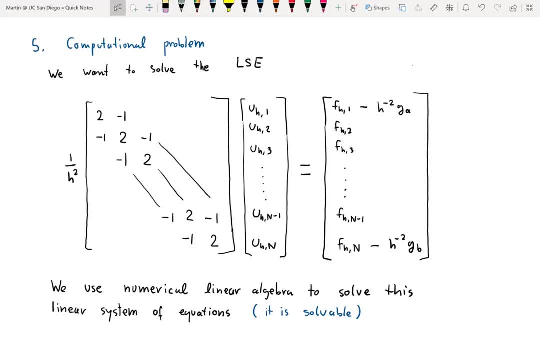 we have got a matrix and a vector of unknowns. The vector of unknowns is very simple. It's uh1,, uh2,, uh3, and so on down to uhn minus 1 and uhn, So the values of the discrete function uh, so to say. 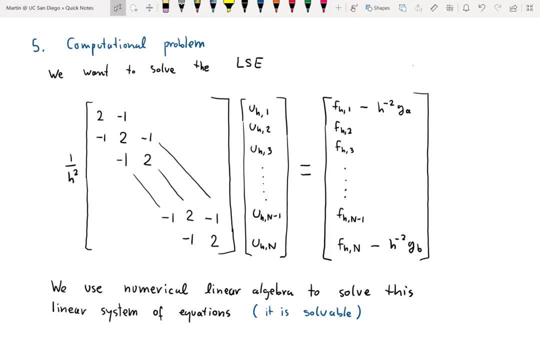 at the interior nodes of the grid are the ones that are in the middle, And then the matrix has a special structure. It's an n times n matrix, of course, And it is tridiagonal. Usually it is written with the vector 1 over h, squared, factored out. 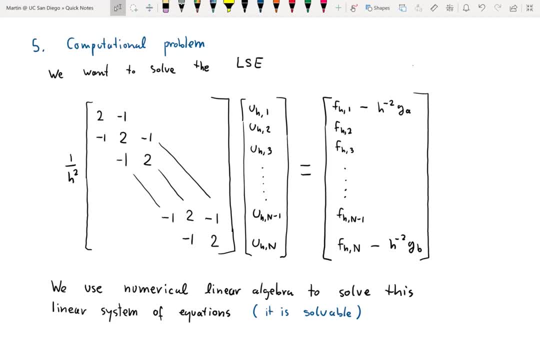 So you can write the matrix compactly as 1 over h squared times the trigonit diagonal matrix, where the main diagonal has only one matrix and the matrix has only one matrix, It has only the value 2 on its entries, and where the upper and lower diagonals 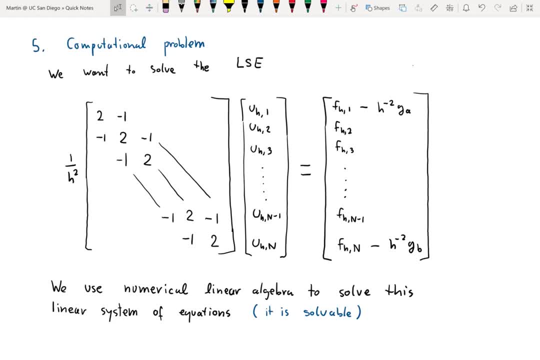 have the value minus 1 in their entries. Okay, that's the linear system of equations, And then we can use techniques from numerical linear algebra to solve this linear system of equations. In fact, we can show that this system is actually solvable. 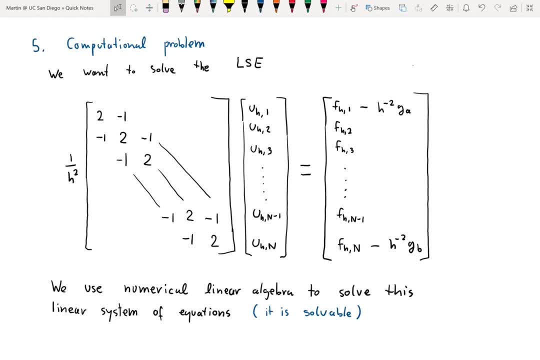 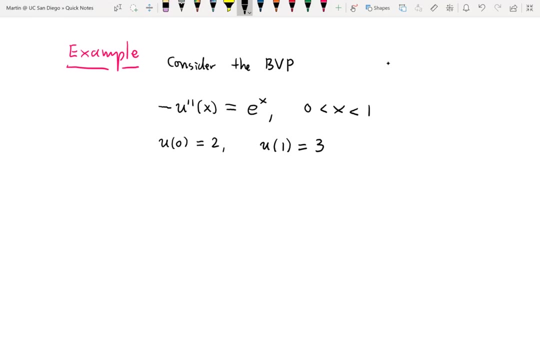 The matrix is invertible, and so for any boundary values and any right-hand side f, we can always get a solution. Now, to round up all this theoretical discussion, let's consider the following boundary value problem Over the interval from 0 to 1,. 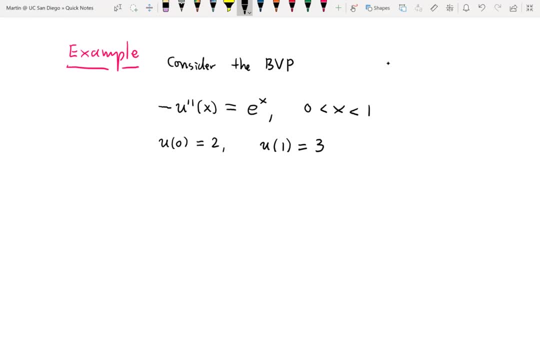 we have the differential equation: u prime, prime of x, equal exponential of x, with the boundary values u at 0 equal 2 and u at 1 equal 3. For the finite difference method, we choose n equal 5.. So we've got 5 interior nodal points. 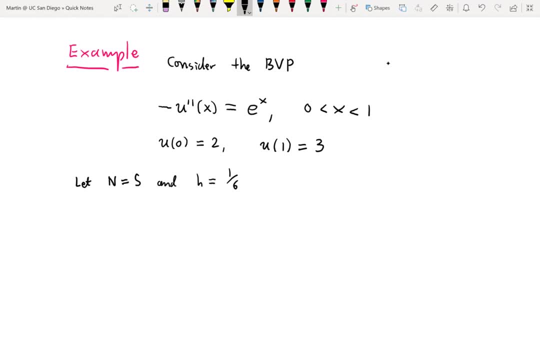 and the step size correspondingly will be 1 over 6.. In total we're going to have n plus 2 nodal points. We have the boundary points x0 and x6, and then the interior nodal points x1, x2, x3, x4, and x5.. 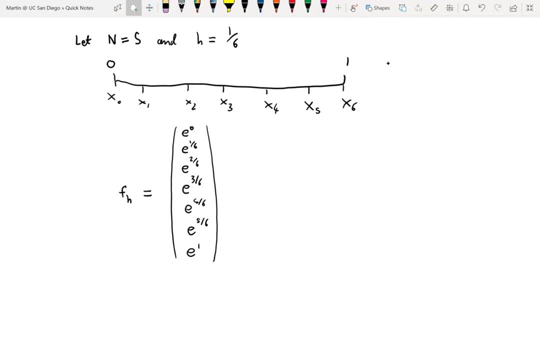 The vector of h is defined as all the values of the function f, which is the exponential function at the different nodal points, So the exponential of 0,, exponential of 1 over 6, exponential of 2 over 6,. 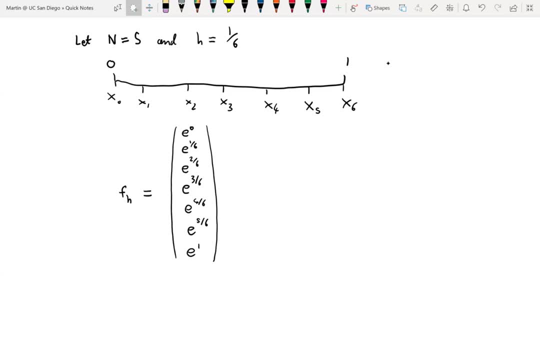 up to exponential of 1.. Nothing very special. Finally, what we get is a linear system in five unknowns and with five equations. The matrix is 1 over 36 times the triad diagonal matrix, with twos on the main diagonal and negative one on the sub- and superdiagonals. 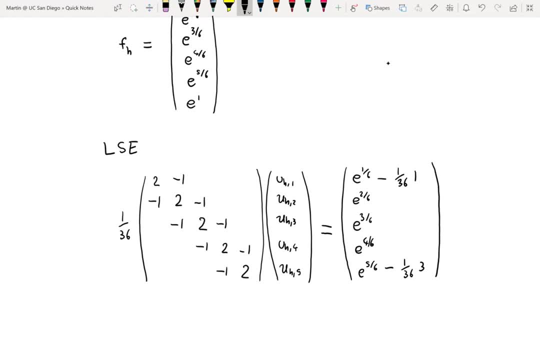 The vector of unknowns contains the variables uh1,, uh2,, uh3,, uh4, and uh5.. And the right-hand side contains exponential of 1 over 6 minus 1 over 36 times 1, exponential of 2 over 6,.